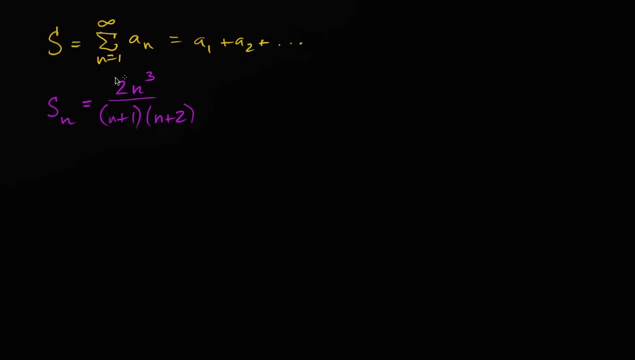 the sum of the first n terms of S is given by this formula right over here. Does this series converge or diverge? Does this thing converge to some finite value, or is it unbounded and does it diverge? Well, one way to think about this. 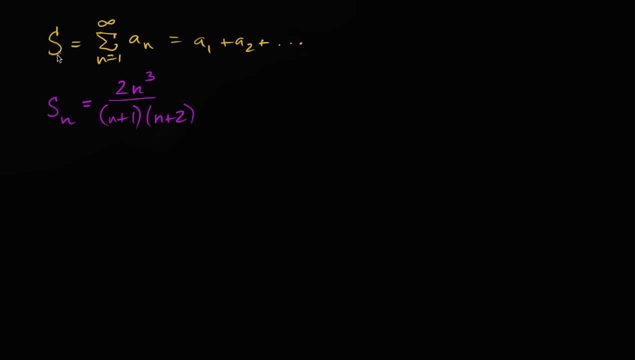 one way to think about this is the idea that our infinite series, S, is just the limit as n approaches infinity of our partial sums. So what do we mean by that? Well, you could imagine a sequence of partial sums here. So you have S sub one, S sub two, S sub three. 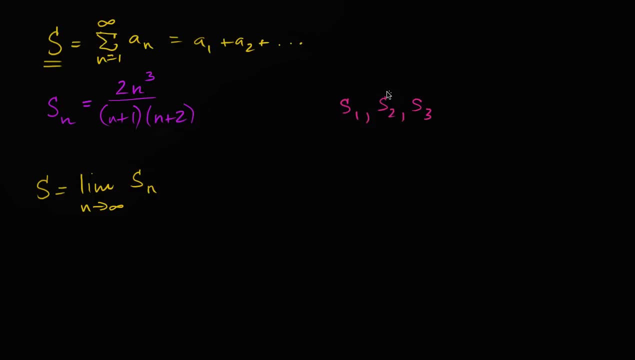 and you keep going going. so this would be the sum of the first term, This would be the sum of the first two terms, This would be the sum of the first three terms, And just think about, well, what happens to the sequence. 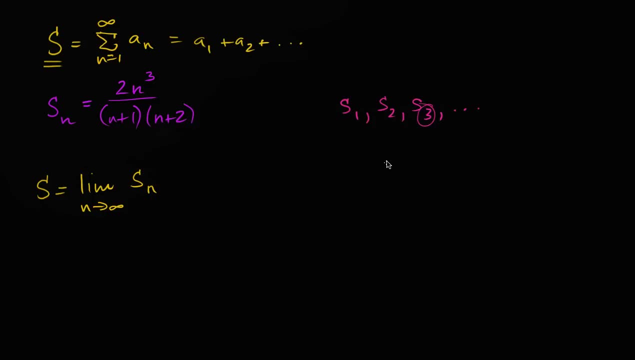 as you go as n as n right over here, approaches infinity, Because that's what the series is. It's the sum of the first- I guess you could say- the first infinite terms. It's the sum of all. you have an infinite number of terms here. 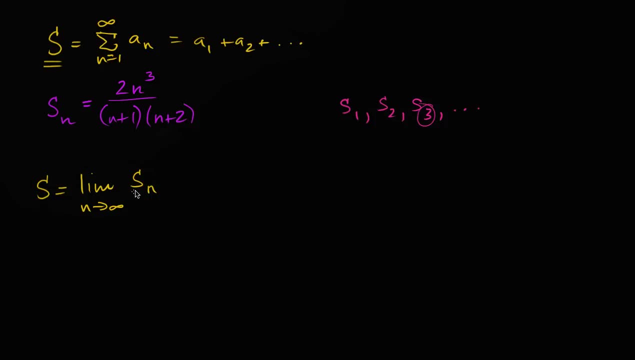 Well, let's think about what this is: The limit as n approaches infinity of s sub n. well, that's just going to be the limit as n approaches infinity of this business right over here. 2n to the third power over n plus 1 times n plus 2.. 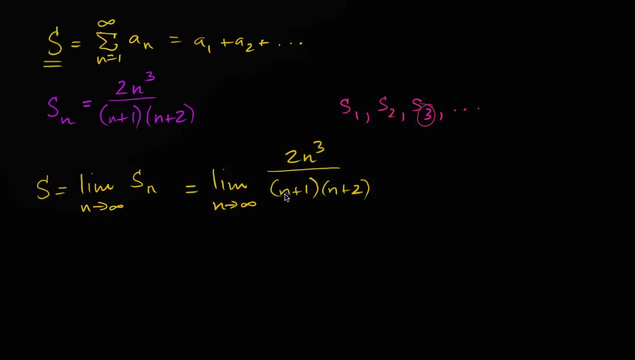 And there's several ways that you could evaluate this. One way you could just realize: hey, look in the bottom, this is going to be a series, This is going to be a second degree polynomial, And up here you have a third degree. 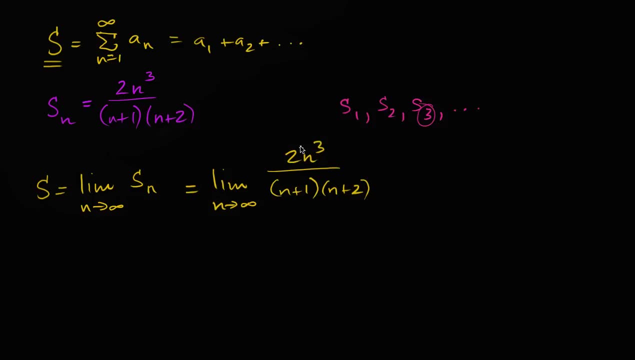 So the numerator is going to grow faster than the denominator, So this is going to be unbounded. So that will immediately tell you. well, this is going to approach infinity, So s is going to diverge, But if you want to do it a little bit, less hand-wavy. 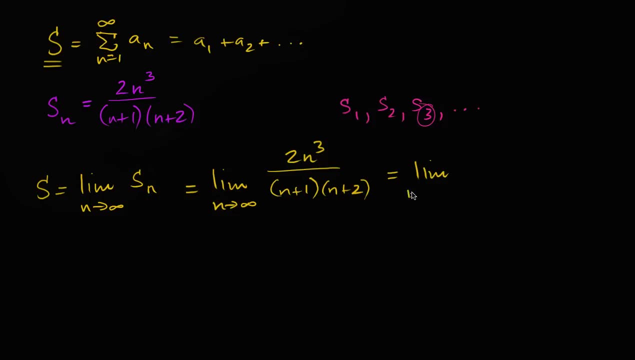 than that. we can actually do a little bit more. algebra Limit: as n approaches infinity, 2n to the third power Over. let's multiply this out: n squared plus 3n plus 2. And let's see we can divide the numerator and the denominator.